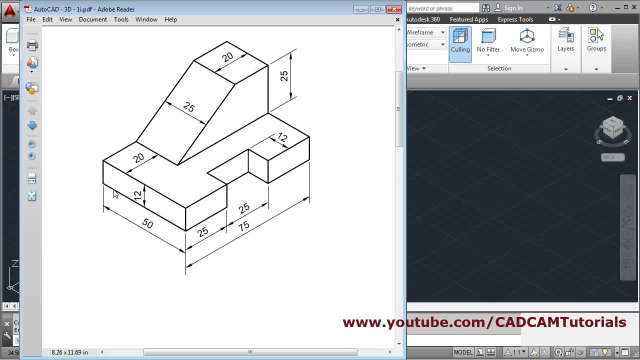 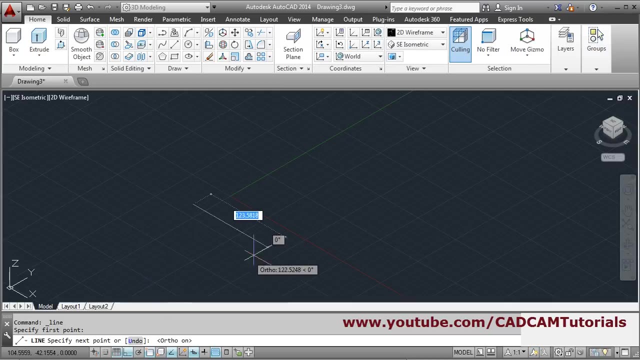 Now in. while creating this object, at first we will create a rectangle of 50 by 75. Then we will press pull it by 12. So first we will take line command, Give first point, make ortho on, Give direction, give distance 50, enter, Zoom it, Then here 75. Then track the end point and connect it. 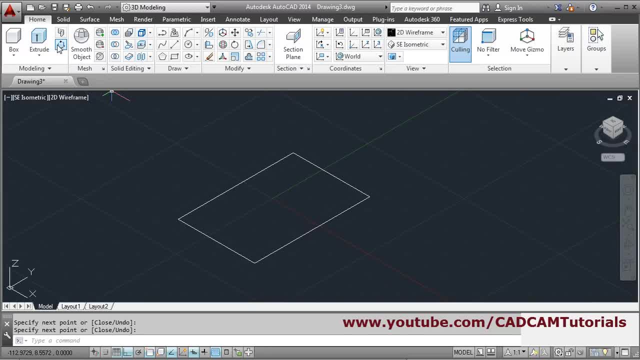 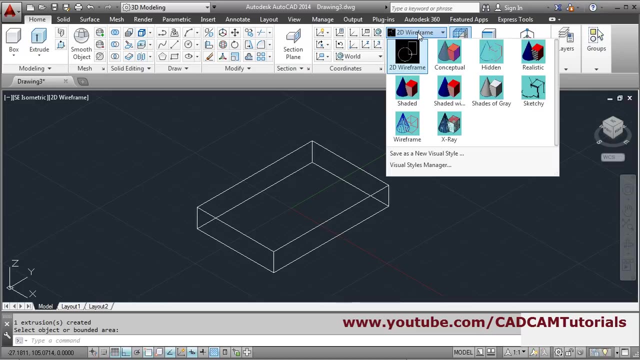 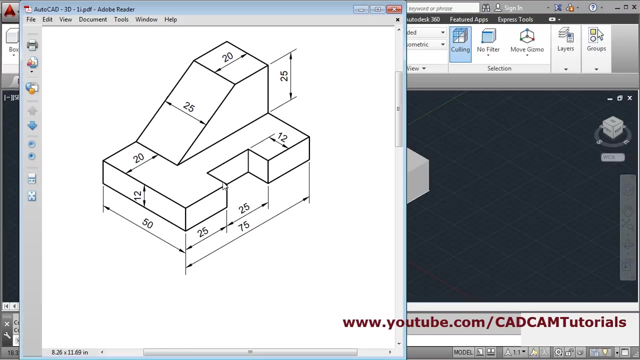 Press enter to come out, Than press pull. Click inside the shape. Give the direction upward, then give the distance of 12.. Press enter to come out To give a 3D look. change the visual style to shaded So it will look like a 3D. Then next we will create this cut. 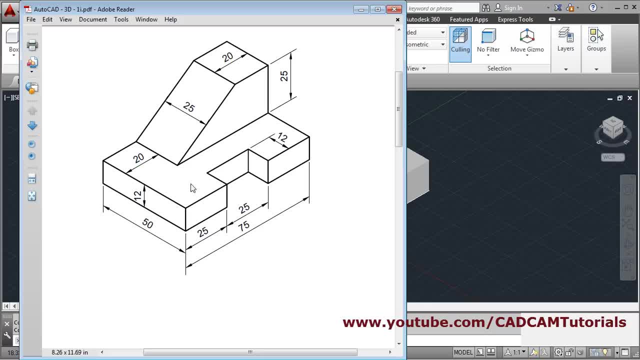 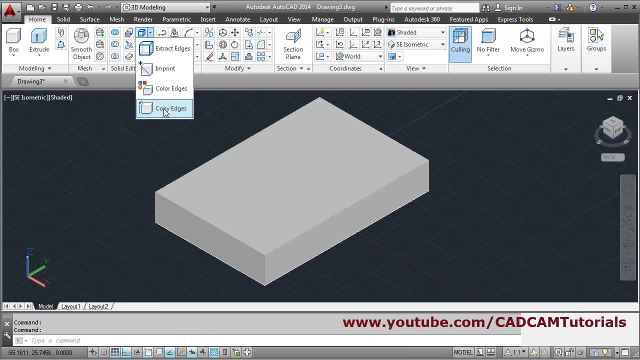 So we will copy this nature action distance of 12.. And this as 3D 25 and 25. so we will use for that from this. extract edges. click on the arrow copy edges will copy this edge. select edge. enter your base point, your. 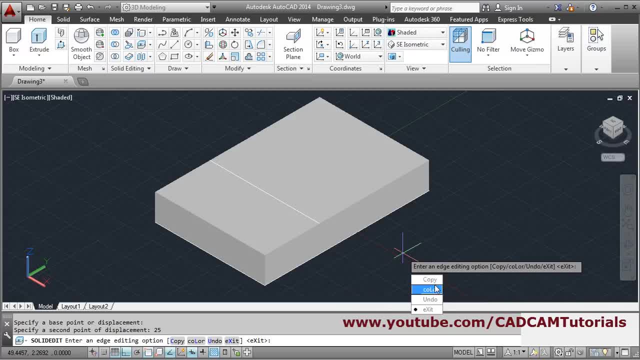 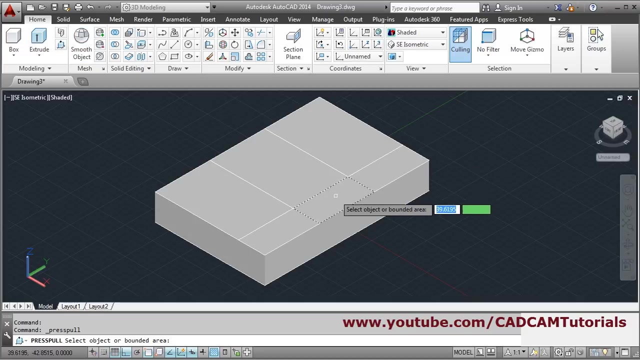 direction and distance of 25. again. copy this edge. enter base point direction and distance 25. again copy this edge. enter base point direction. distance of 12. enter exit. click on exit to come out. then we will cut this shape using press pull. so press pull, go inside the shape, click there, give the direction. 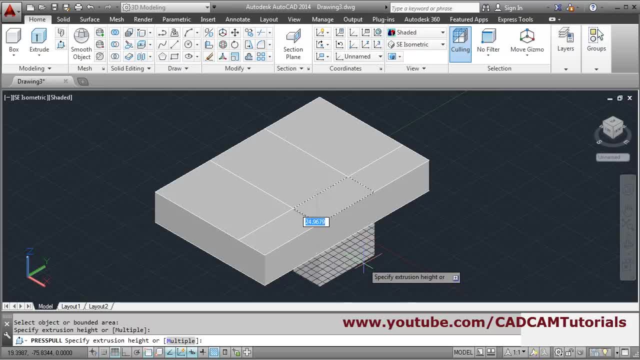 below and you can either give the dimension or you can click there also so it will cut it. press enter to come out unwanted object. you can erase it. so you just enter and select the unwanted object. so by making an exit we will get the shape of this object, so we will cut this shape. 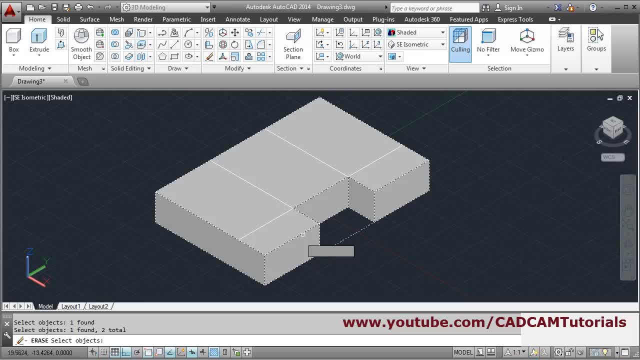 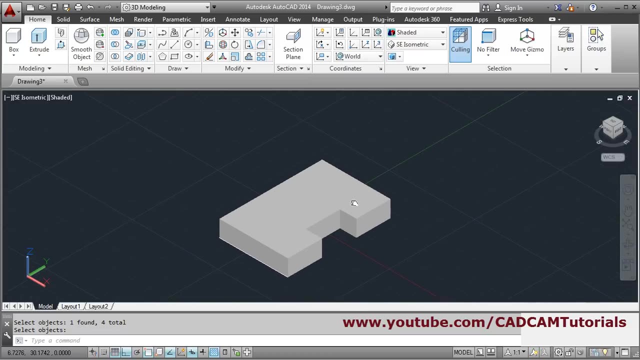 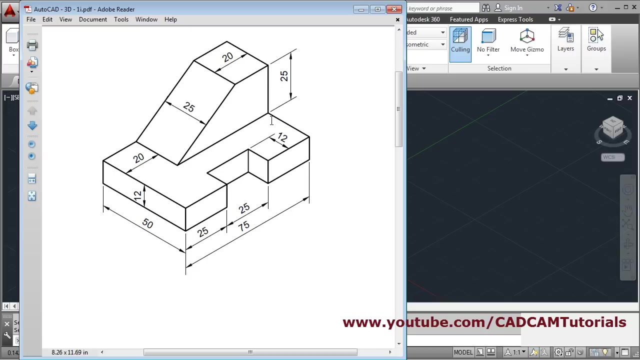 mistake. actually this 3d object is selected. if you want to cancel the selection, just hold down the shift and click on the 3d object. it will cancel the selection. so just select these lines, press enter, so it will. it is unwanted objects. then next we will have to create this shape. now we will create this shape. 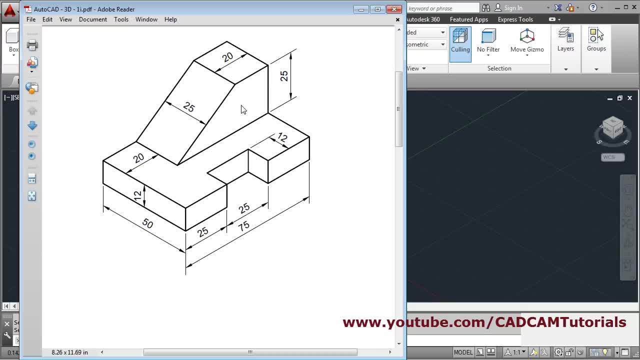 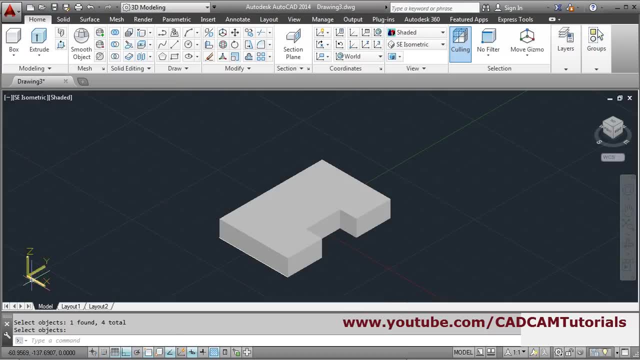 and press pull this in this direction. so we have to change the direction of Zed, actually, because press pull is always carried out in Zed direction. now Zed is vertical. therefore it was press pulled in vertical direction, but we want to go horizontal in this direction. therefore, we will change the UCS to: 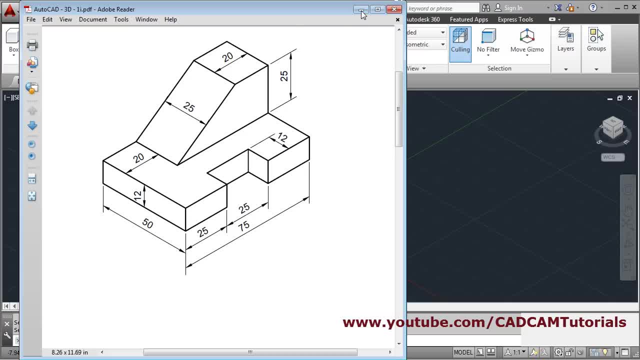 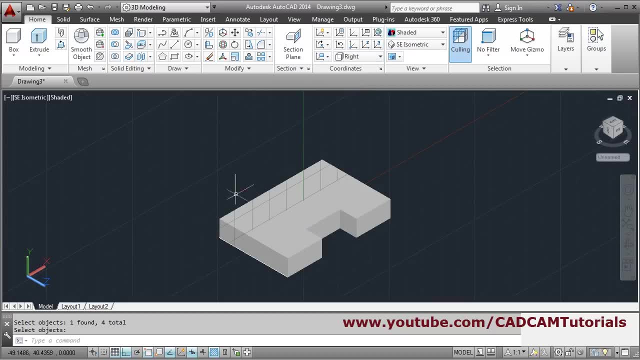 matching this up so we will take the right UCS. so from here we will change the UCS to right. then this grid are coming inside, so we will just obviously change the direction of the grid grid display. then on right side we will create the shape. this shape, that is, this, is of 55, 25, 20. so we will again take a. 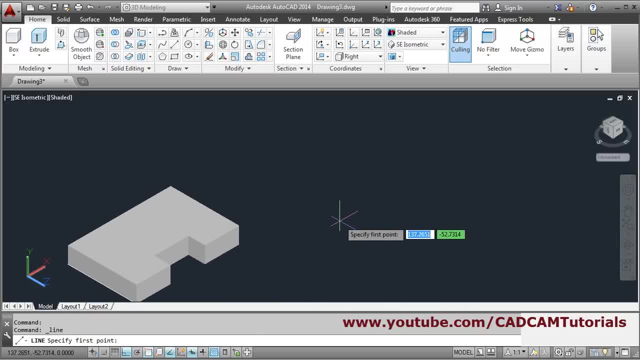 line: give the. we will create it outside. so principle will be easy. first point: give the distance of 55, go vertical. give distance of 25, then come down side Q distance of 20. connect it to the end point, enter, then again press, pull it, so will press put. 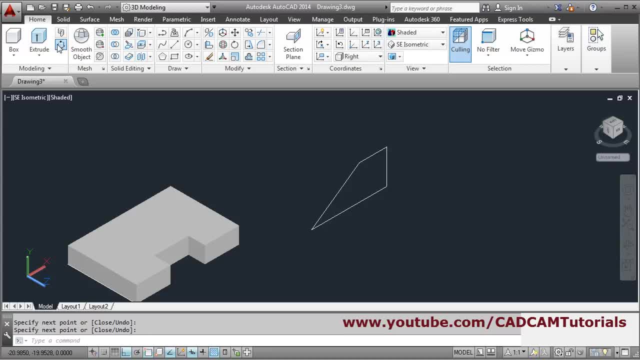 it a, press fully by 25. so preschool: click inside the object, give the direction Q the distance of 25, press ENTER. press ENTER to come out. then you can move this object. move, select object, enter. then actually we will need a backward end point. so we will just. 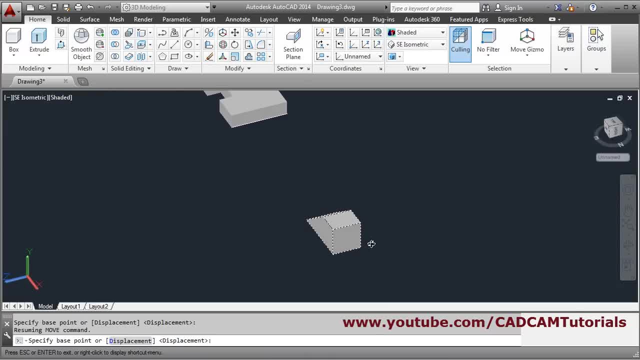 orbit it by holding down the shift and scroll, and then we will take this as a base point and second point will be this one. so we will come back to original view by clicking on this AC isometry. then we can erase it by giving a enter select. 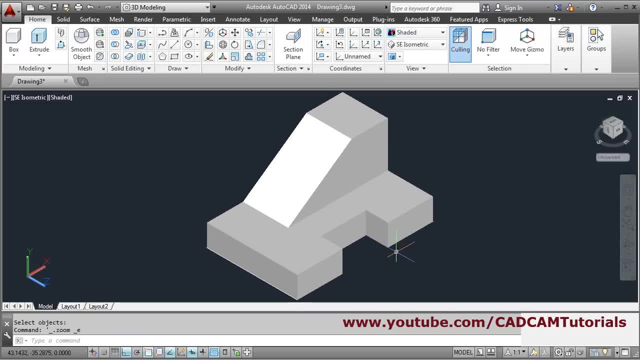 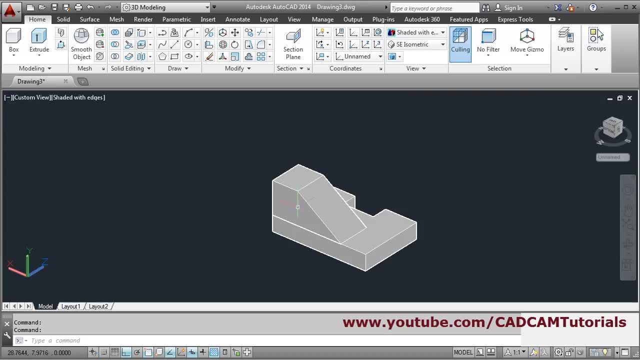 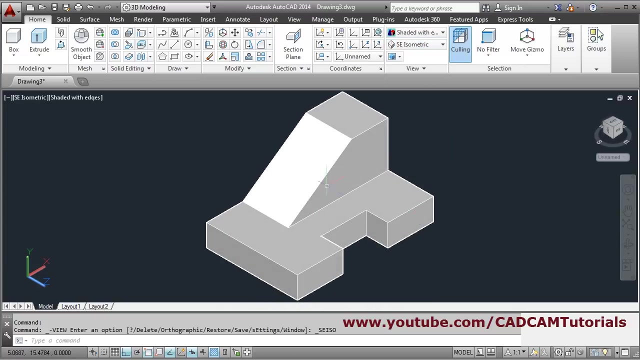 the by crossing window, so this object is created. but but if we view this object in shaded with edges? so these are two separate objects. so we can connect them using union command- here solid union- click on both the object, press enter, so it will be merged into each other again. click on AC isometry: same this way we. 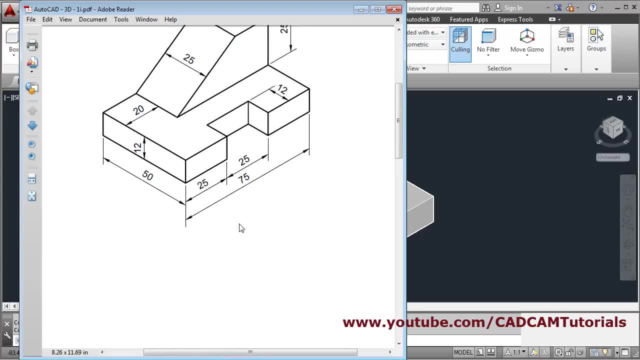 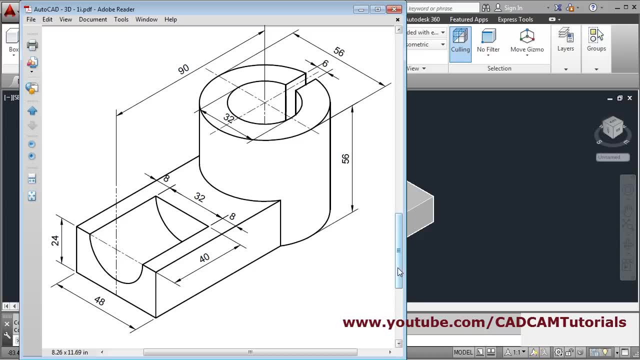 created this object, the next object will be this one. suppose we want to create this object. so for this also again, we will take 150 view 150 as a limit. so we will take 150 view 150 as a limit. so for this also again, we will take 150 view 150 as a limit. so for this also again, we will take 150 view 150 as a limit. 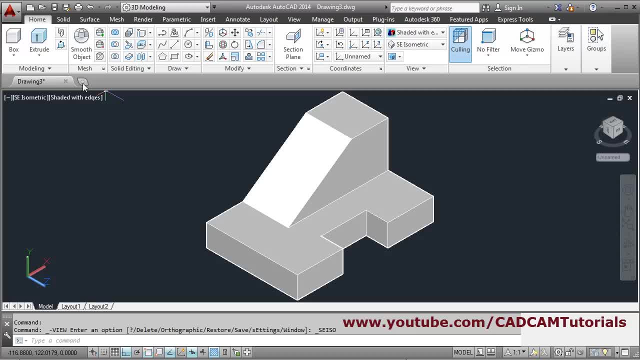 so again, we will take 150 view 150 as a limit. so for this also, again, we will take 150 view 150 as a limit. so again, I will click on this to start a new. so again, we will take 150 view 150 as a limit. so again, I will click on this to start a new. 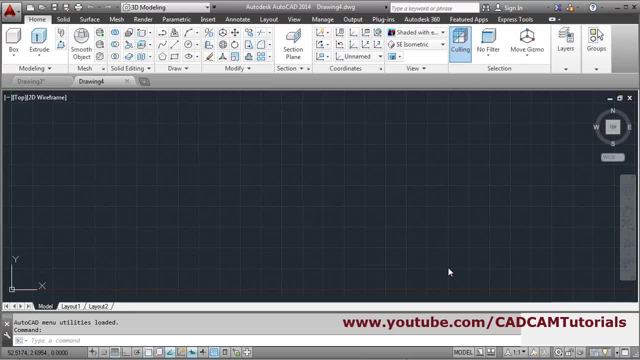 so again, we will take 150, view 150 as a limit. so again, I will click on this to start a new drawing. a CAD open again. I will, from here I drawing a CAD open again. I will, from here I, drawing a CAD open again. I will, from here I will switch to this. okay, before that I 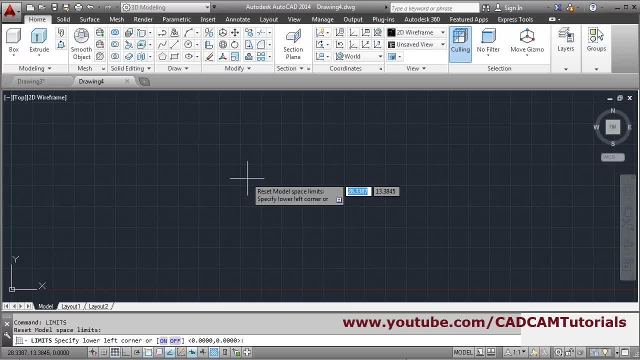 will switch to this. okay, before that I will switch to this, okay, before that. I will set the limits 0 comma 0, then will set the limits 0 comma 0, then will set the limits 0 comma 0. then suppose: 200 comma 200 enter. Z enter. enter. 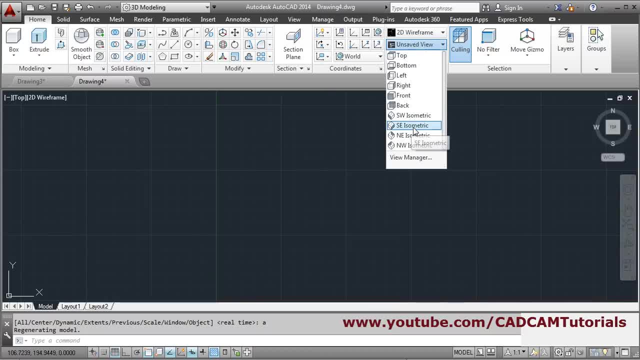 suppose 200 comma 200, enter Z, enter- enter. suppose 200 comma 200, enter Z- enter, enter for zoom. or then change the visual for zoom, or then change the visual for zoom, or then change the visual. style is a symmetric, then again UCS icon. style is a symmetric, then again UCS icon. 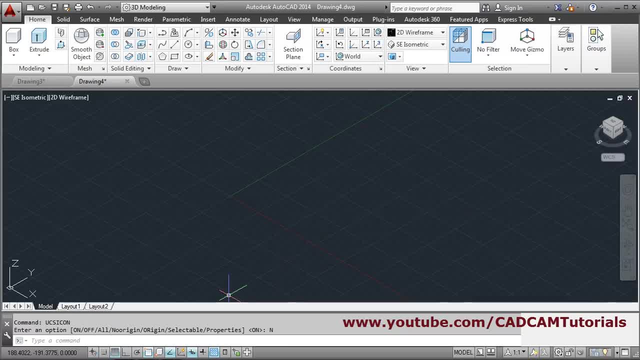 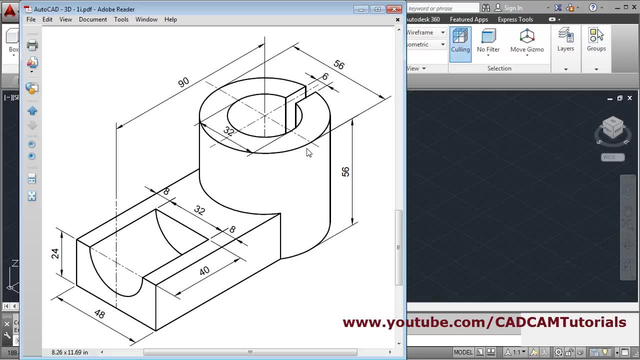 style is a symmetric. then again UCS icon: enter no region, then creating this: enter no region, then creating this: enter no region, then creating this object. so at first we will create suppose object. so at first we will create suppose object. so at first we will create, suppose this circle 56 diameter and 32 diameter. 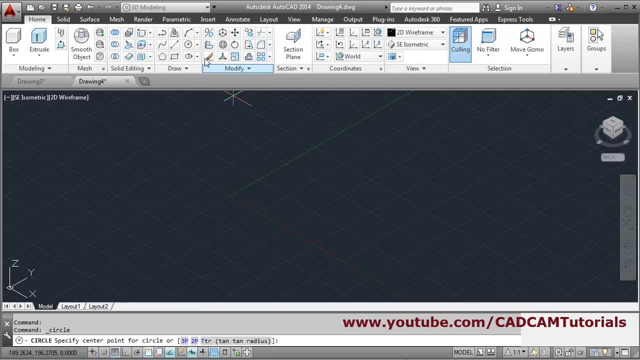 this circle 56 diameter and 32 diameter. this circle 56 diameter and 32 diameter. so take circle command. okay, we will take. so take circle command, okay, we will take. so take circle command, okay, we will take. suppose diameter option Center point. suppose diameter option Center point. 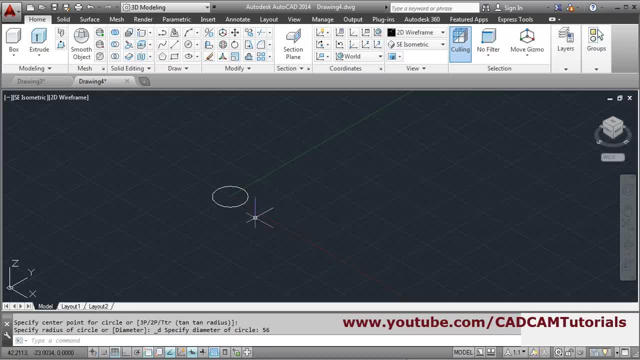 suppose diameter option, Center point. give the diameter of 56, give the diameter of 56, give the diameter of 56, zoom there again. circle same diameter option. zoom there again, circle same diameter option. zoom there again circle- same diameter option. give the center distance of 32, then 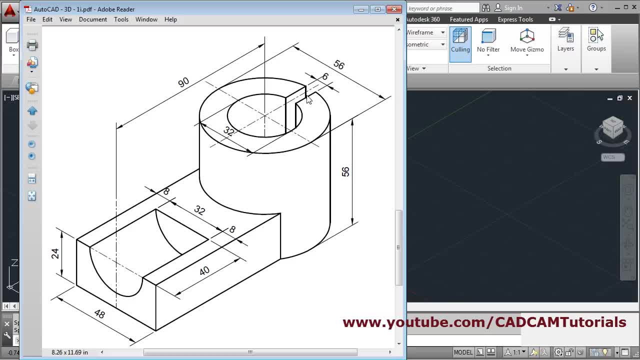 give the center distance of 32, then give the center distance of 32, then next is one cut is there of 6 distance. next is one cut is there of 6 distance. next is one cut is there of 6 distance from Center. so we will offset it and 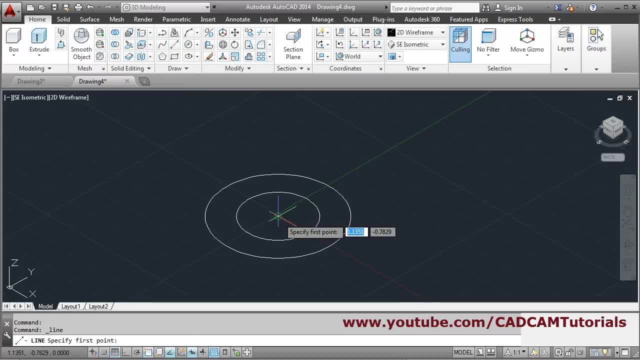 from Center, so we will offset it, and from Center, so we will offset it and create that. so take line command. take, create that. so take line command. take, create that. so take line command. take the reference from the center and create the reference from the center and create. 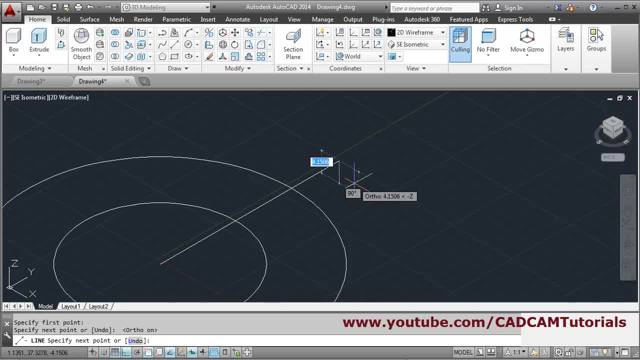 the reference from the center and create one line again. make or throw on. click one line again. make or throw on. click one line again. make or throw on. click outside. press enter then offset this outside. press enter, then offset this outside. press enter, then offset this line. offset by distance of 3. select this. 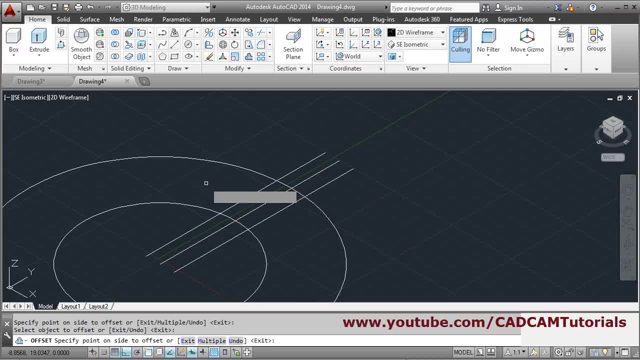 line offset by distance of 3. select this line offset by distance of 3. select this line on this side. select this line on line on this side. select this line on line on this side. select this line on other side. click there, press enter. then other side: click there, press enter then. 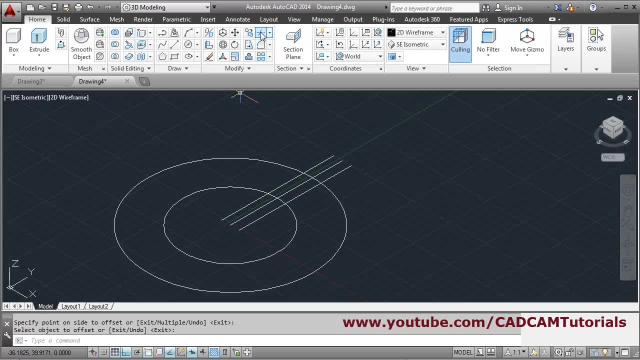 other side, click there, press enter, then trim the unwanted objects. so just use, trim the unwanted objects, so just use, trim the unwanted objects, so just use here trim. so I will take, suppose this as here trim. so I will take, suppose this as here trim. so I will take, suppose this as a cutting edges, then enter, then cut the. 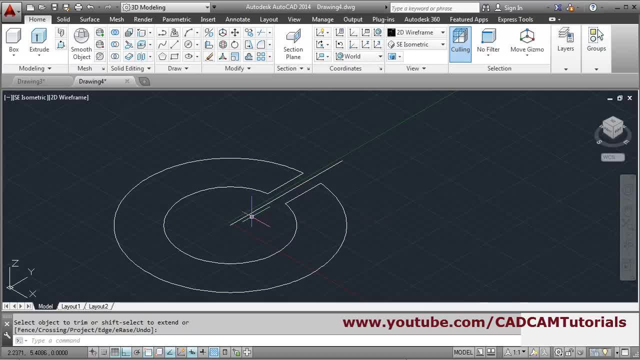 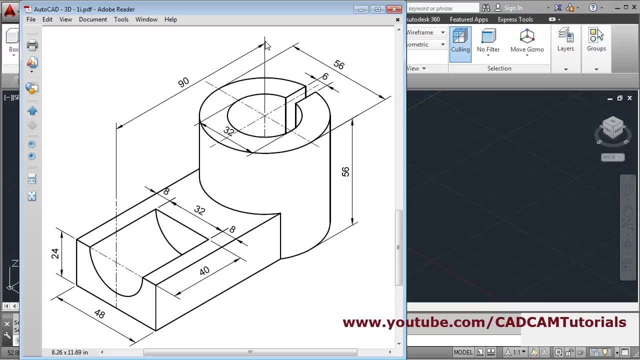 and we can remove this line by erase command. so this shape is created. this rectangle is to be created at a created. this rectangle is to be created at a created. this rectangle is to be created at a distance of 90 distance, so we will. distance of 90 distance, so we will. 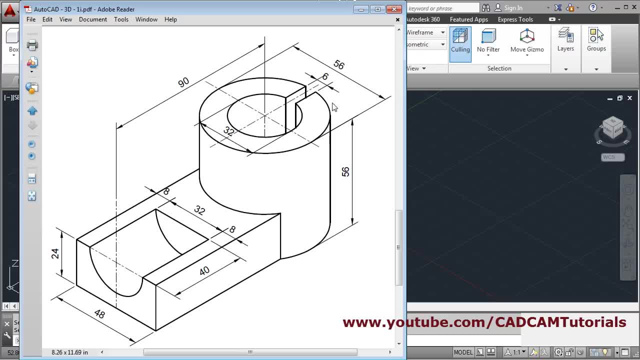 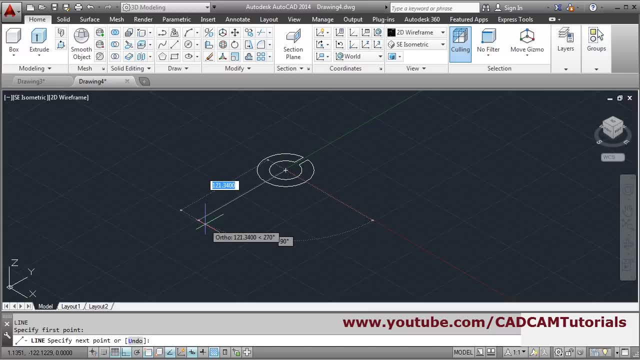 distance of 90 distance. so we will just create one line from here from the, just create one line from here from the, just create one line from here from the center at a distance of 90, distance of center, at a distance of 90, distance of center at a distance of 90, distance of 90 line. then 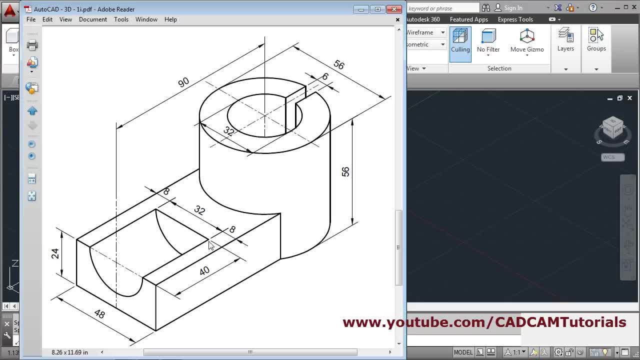 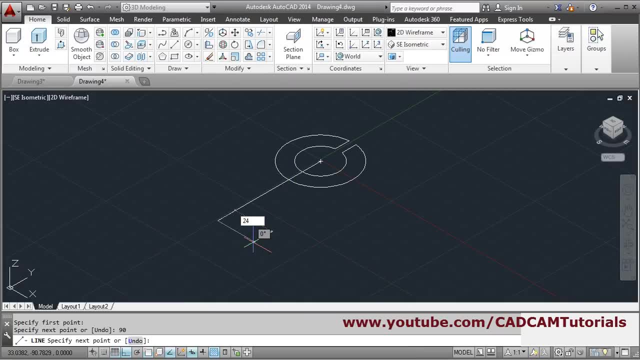 90 line, then 90 line, then from here I have to: the width is 48, so 24. from here I have to: the width is 48, so 24. from here I have to the width is 48, so 24 on either side. so here 24 and here it. 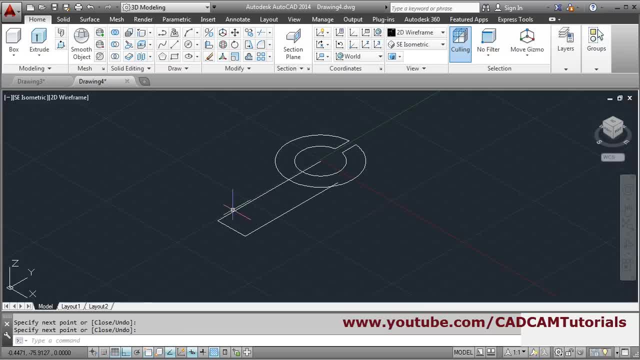 on either side. so here 24, and here it on either side. so here 24, and here it will touch the circle, and then we can will touch the circle, and then we can will touch the circle and then we can mirror this. so we'll use the mirror. 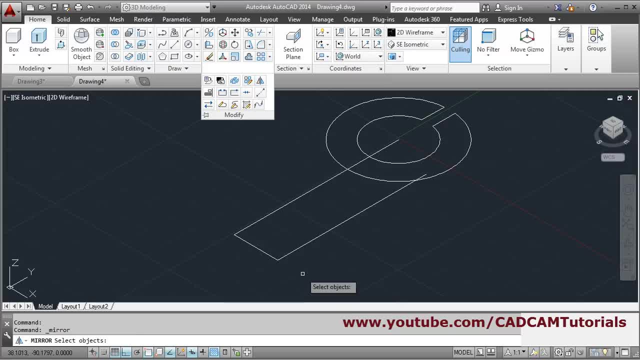 mirror this. so we'll use the mirror mirror this. so we'll use the mirror command 2d mirror. so here is the mirror command 2d mirror. so here is the mirror command 2d mirror. so here is the mirror. select both the object enter. 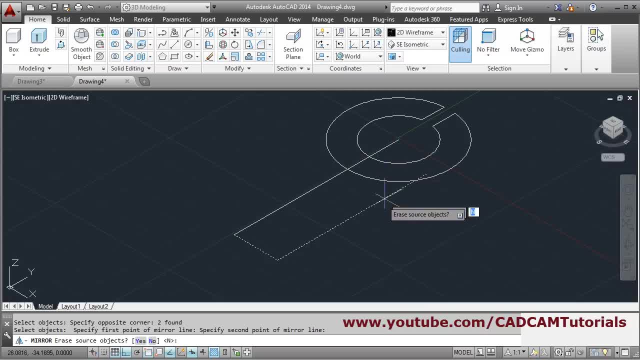 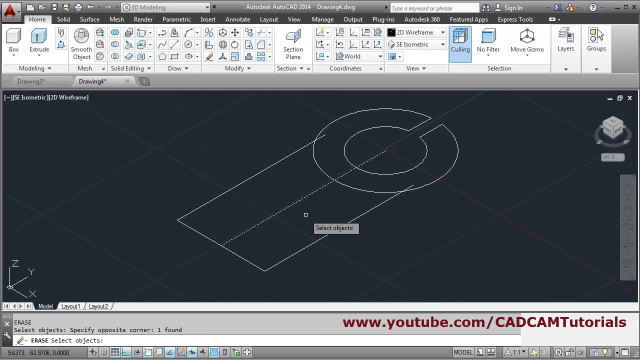 select both the object enter and select both the object enter and mirror line will be this one first point. mirror line will be this one first point. mirror line will be this one first point. second point for the mirror line, then second point for the mirror line, then second point for the mirror line, then enter, then again erase this. he enter. 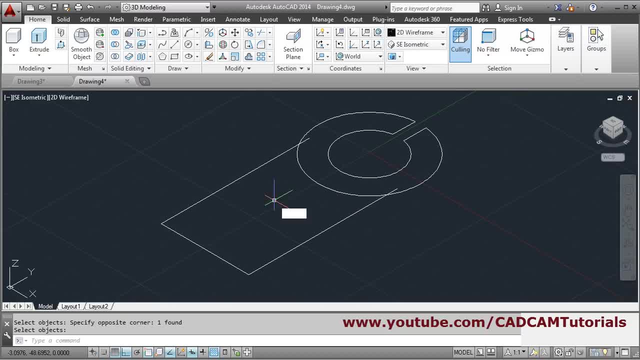 enter, then again erase this. he enter. enter, then again erase this. he enter. select the object. press enter again trim. select the object. press enter again trim. select the object. press enter again trim. you can by typing TR. you can use the. you can by typing TR. you can use the. 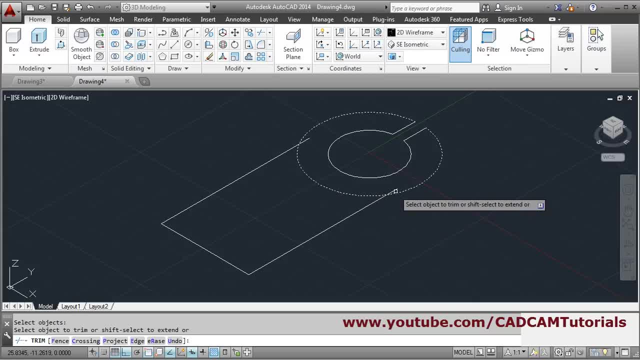 you can by typing TR. you can use the trick trim command: select cutting edges. trick trim command- select cutting edges. trick trim command- select cutting edges- enter. select the unwanted object. so this enter. select the unwanted object. so this enter. select the unwanted object. so this piece work is ready. then we will press. 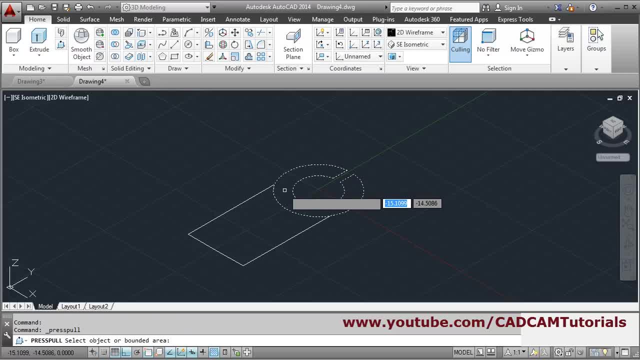 piece work is ready, then we will press. piece work is ready, then we will press. pull it, press pull. go inside the shape. pull it- press pull. go inside the shape. pull it- press pull. go inside the shape. give the height of 56 press enter I can. give the height of 56 press enter I can. 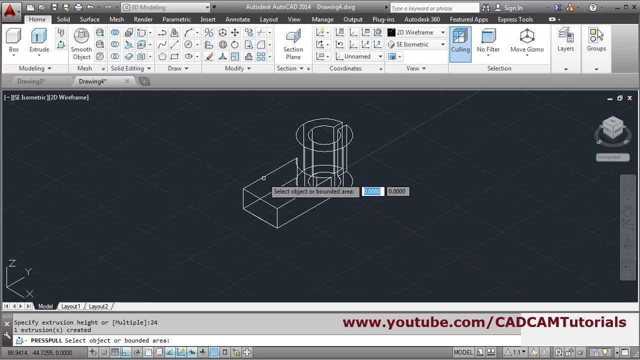 give the height of 56. press enter. I can go inside here again. height of 24. go inside here again. height of 24. go inside here again. height of 24. press enter to give a 3d look. change the. press enter to give a 3d look. change the. 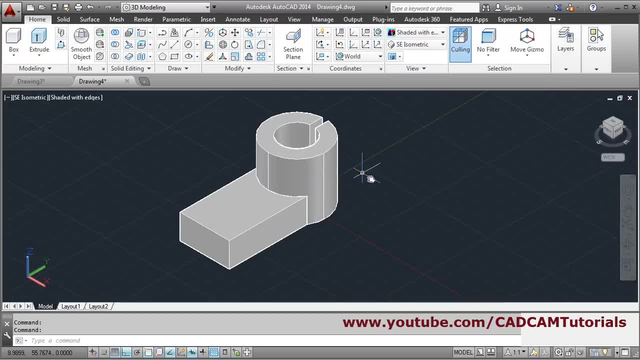 press enter to give a 3d look. change the visual style to share it with ages. so in visual style to share it with ages. so in visual style to share it with ages. so in this way this object is created then this way this object is created then. 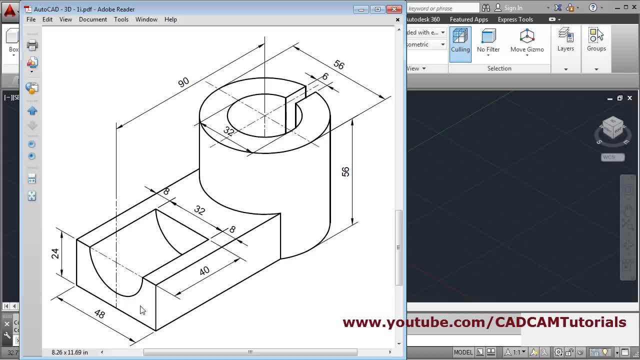 this way this object is created, then this cut so 32 is the radius of this. this cut so 32 is the radius of this. this cut so 32 is the radius of this circle. again, we have to create a circle. circle. again, we have to create a circle. 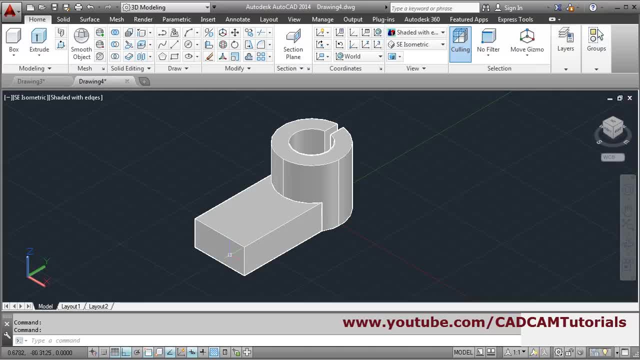 circle. again, we have to create a circle on this plane. so we will change the UCS on this plane. so we will change the UCS on this plane. so we will change the UCS icon to front plane. so from here we will. icon to front plane. so from here we will. 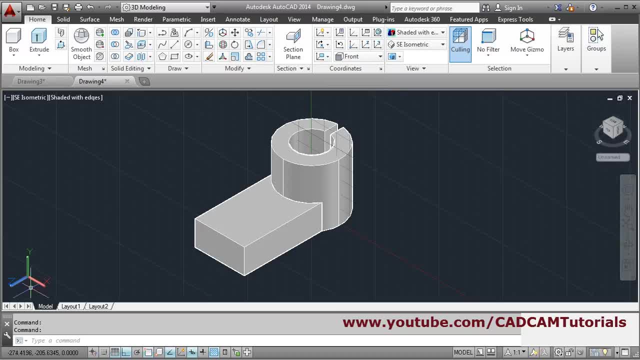 icon to front plane. so from here we will change the front plane to front again- XY. change the front plane to front again- XY. change the front plane to front again. XY is parallel to this one again. from is parallel to this one again. from is parallel to this one again. from. circle Center. diameter is the center. 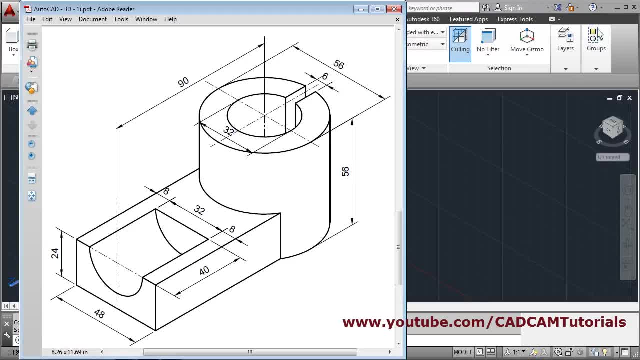 circle Center diameter is the center circle Circle Center diameter is the center point, then 32 is the diameter. so point then 32 is the diameter, so point then 32 is the diameter. so give the 32 enter zoom there now this grid. give the 32 enter zoom there now this grid. 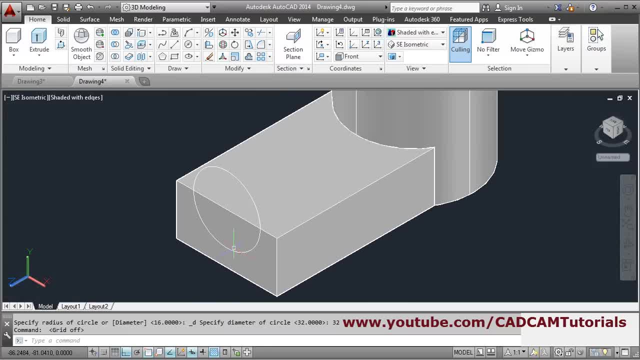 give the 32 enter zoom there now this grid are coming inside, so we will of the are coming inside, so we will of the are coming inside, so we will of the grids. then again, use the press, pull go grids. then again, use the press, pull go grids. then again, use the press, pull go inside the shape you want to cut give. 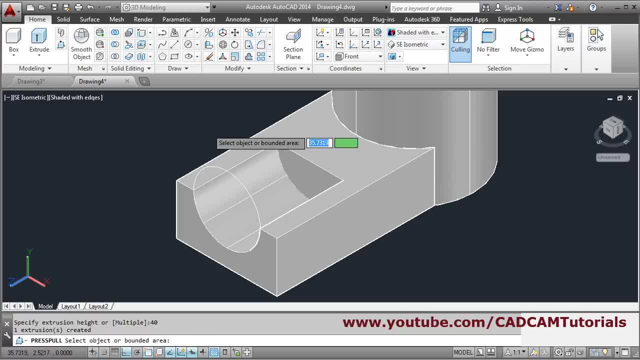 inside the shape you want to cut, give inside the shape you want to cut, give the direction and give it the distance, the direction, and give it the distance, the direction, and give it the distance of 40 press enter to come out. it is this: of 40 press enter to come out, it is this: 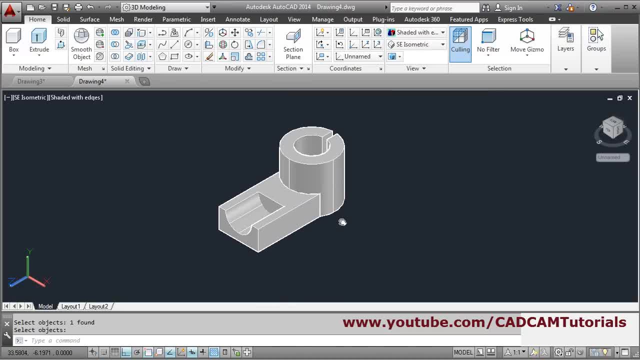 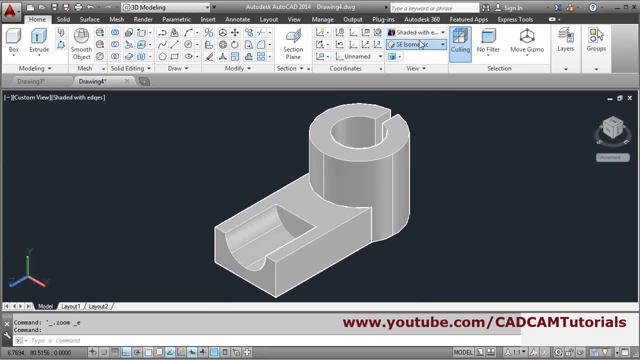 of 40. press enter to come out. it is this circle enter. click on the circle. press circle enter. click on the circle press circle enter. click on the circle. press enter. so in this way this object is enter. so in this way this object is enter. so in this way this object is created. click on its asymmetry if you. 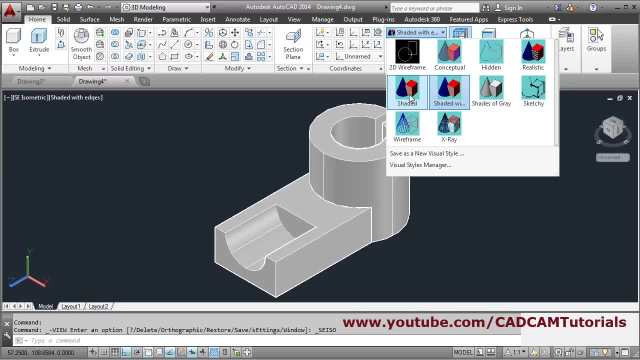 created, click on its asymmetry. if you created, click on its asymmetry. if you don't want to see these lines, you can don't want to see these lines. you can don't want to see these lines- you can click on shade it. and if you want to use,